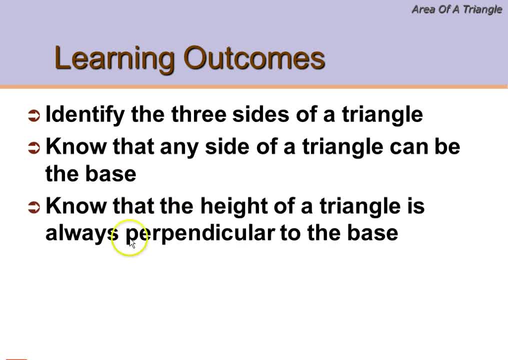 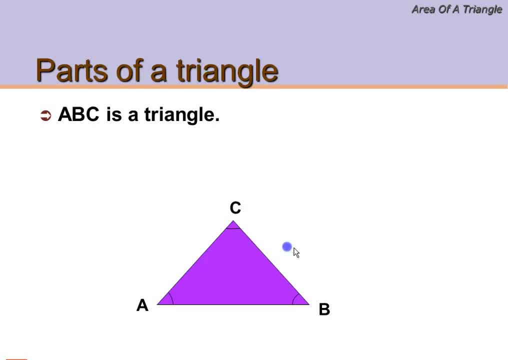 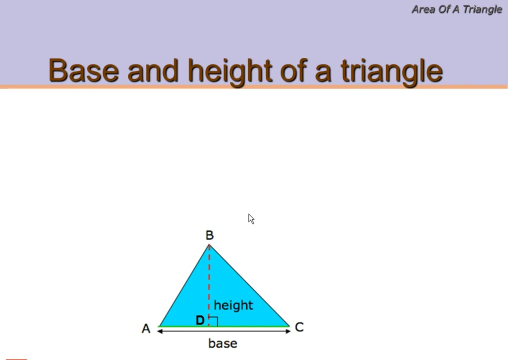 Know that the height of a triangle is always perpendicular to the base. In triangle ABC it has three sides and three angles. Right, the sides are ABC, B, BC and CA. In this triangle, BD is perpendicular to AC. AC is the base of the triangle and BD is the height of the triangle. 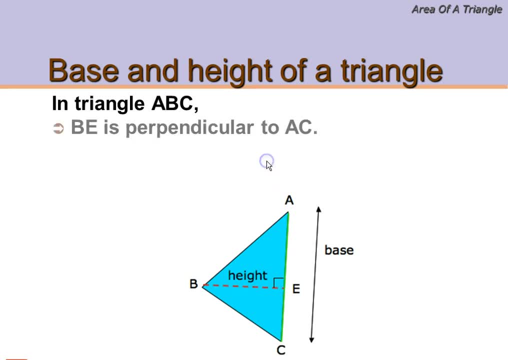 In this similar triangle, BE is perpendicular to AC. AC is the base of the triangle and BE the height In this triangle. ABC, CF is perpendicular to AB. AB is the base, CF is the height. In triangle PQR, the base is QR and the height is PS. 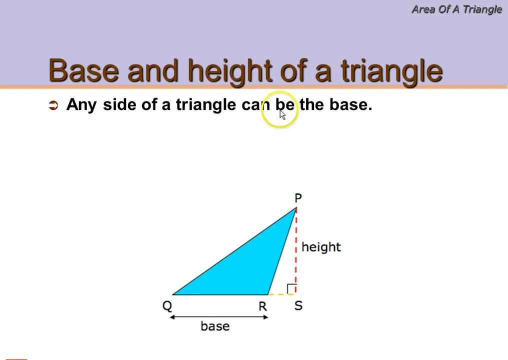 Kindly note that any side of the triangle can be the base. The height must always be perpendicular to the base. Hence, in this triangle, PQR, QR is the base and PS the height. PR is the base for this triangle, PQR and QT is the height. 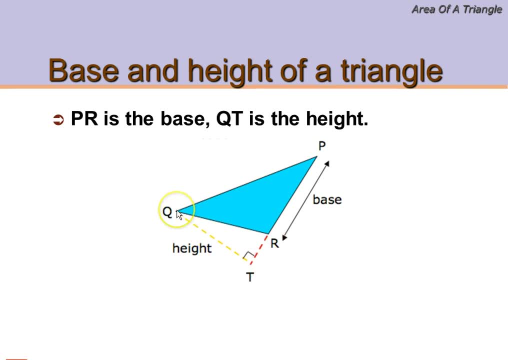 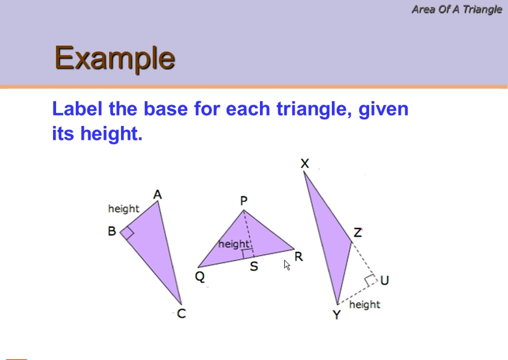 not QR. QT is perpendicular to TR and also to PR. QP is the base and RU the height Label, the base for each triangle, given its height. AB is the height, PS is the height And YU is the height. Where are the bases?